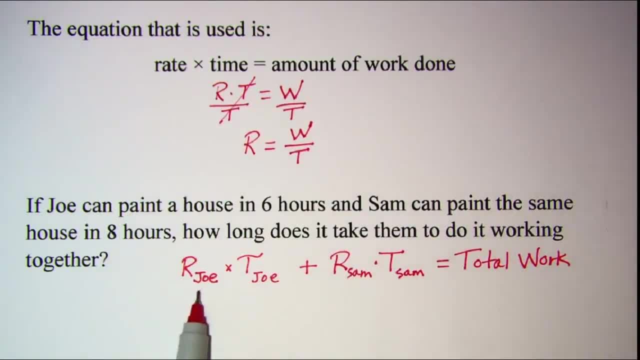 So the first average rate equals the amount of work done by Sam, which is 1-10.. When Joe added times' time, Sam added no work. When Joe added times' time' Sam added no additional work And Sam added no additional work. 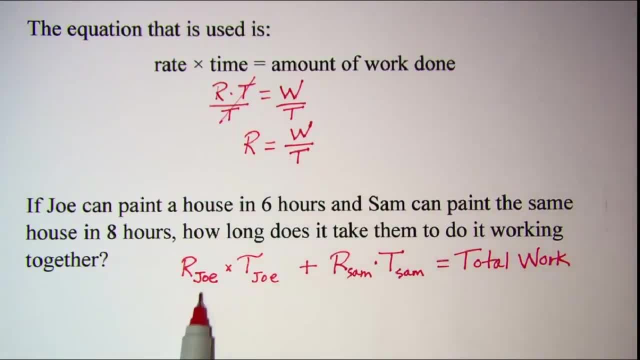 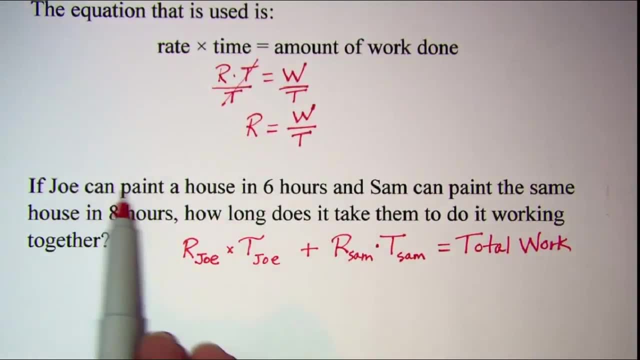 So if you clumsy mistake to always leave the神 rate and thestaw rate completely unchanged in our equation, then we'll do the same thing for Sam and Joe. We'll take this first sentence. It says: Joe can paint a house in six hours. So a house, basically just one house. 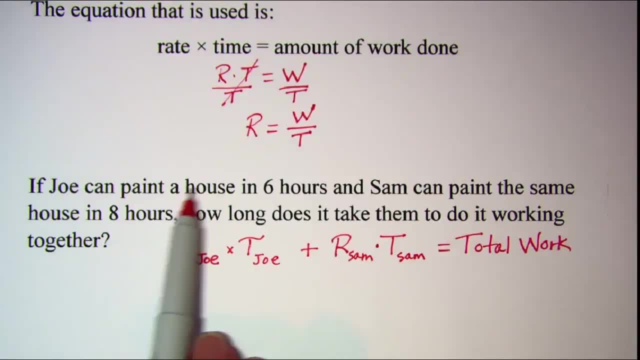 So we have one house is the amount of work done and six hours is the time. So Joe's rate is one sixth. Or if you wanted to talk about in terms of rate, you could say one sixth of the house per hour. So one house in six hours And then we'll be multiplying that by Joe's time. 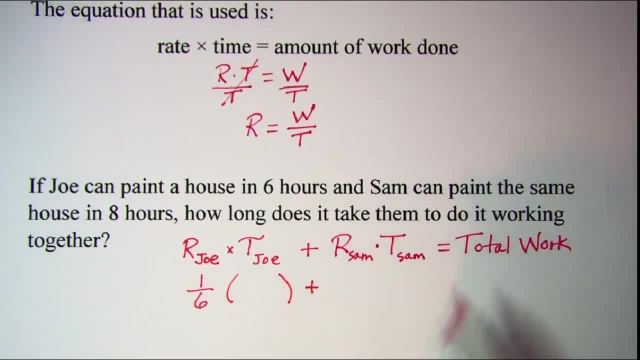 I'm going to wait for a minute and put that in after we finish the rates, Sam's rate. We'll take the second part of this first sentence here. Sam can paint the same house, So one house in eight hours. So Sam's rate is one house in eight hours, or one eighth of a house per hour. 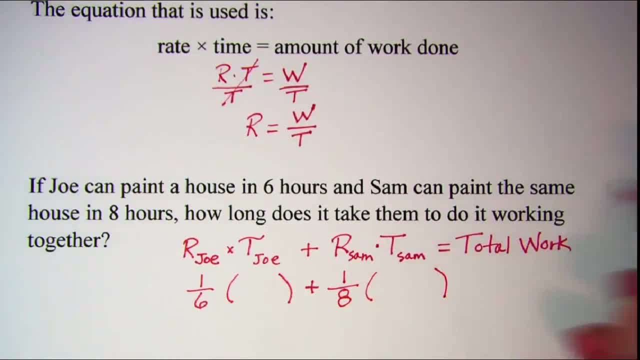 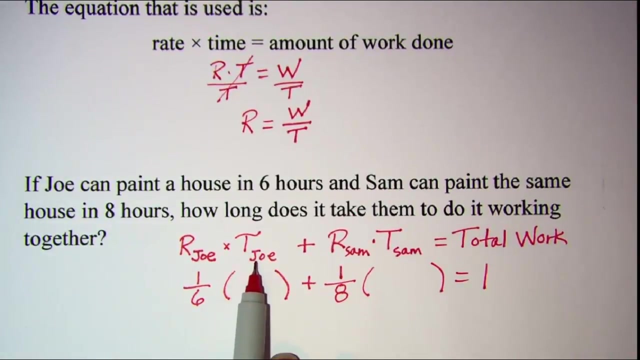 And then we'll multiply that by Sam's time and the total work that they have to get done together. How long does it take them to do it? So painting one house. So our total work is going to be one house. Now we need our times for the both of the men. 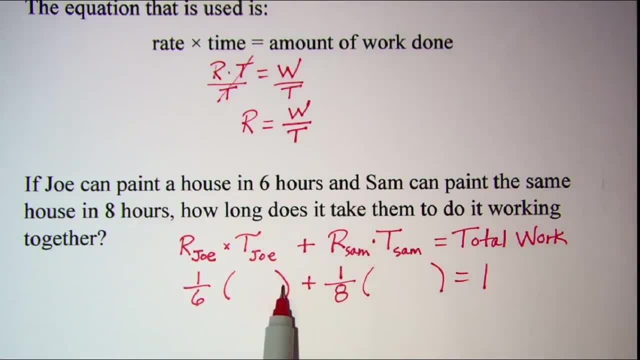 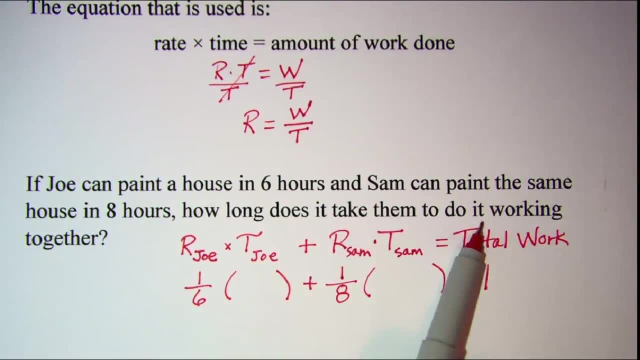 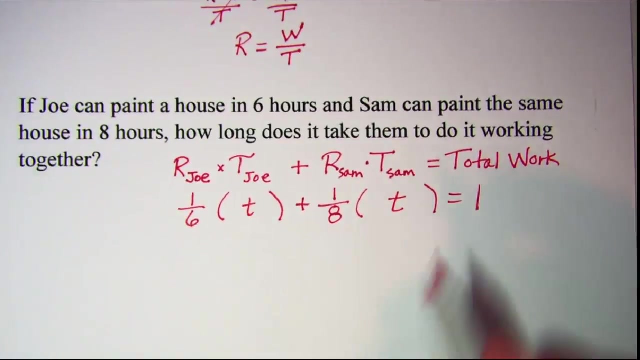 How long does it take them? So we're basically looking for the time. We're assuming that they're starting at the same time and finishing at the same time because they're working together. So we'll just let the time for both men be t.